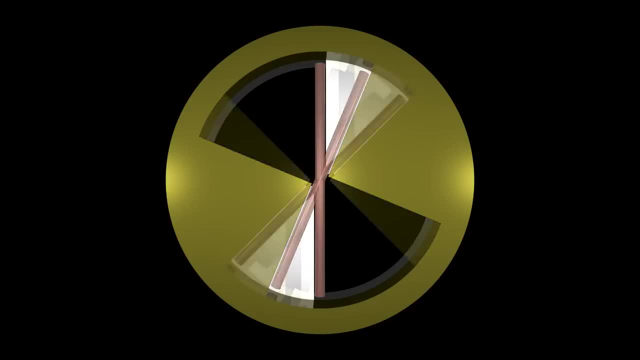 Here's the range for pass B- fail C And here's the range for pass A- fail C. We can see that the probability to pass A and fail B plus the probability to pass B and fail C is equal to the probability to pass A and fail C For this cartoon experiment. 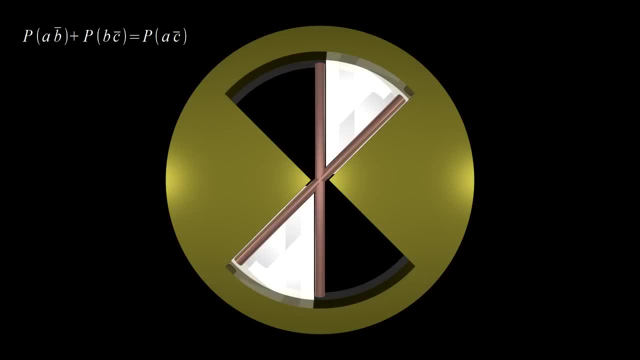 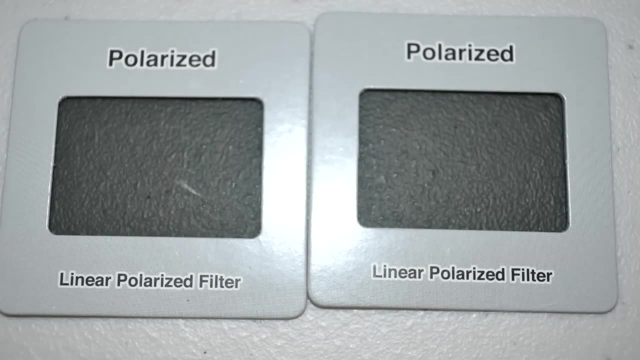 Bell's inequality is satisfied in its equality form. In the real world, Bell's inequality is obvious. Bell's inequality is the probability that a rod will pass the first test and fail the second test. In the real world, Bell's inequality is often tested using photons and polarization filters. 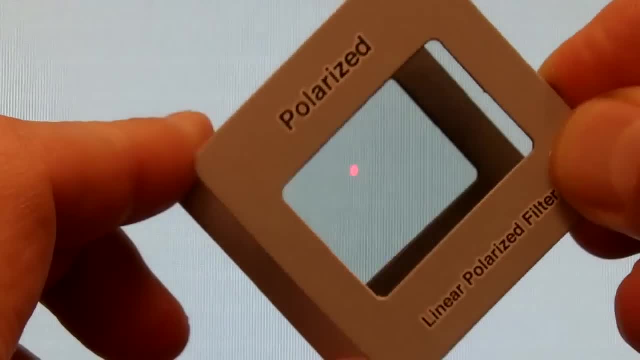 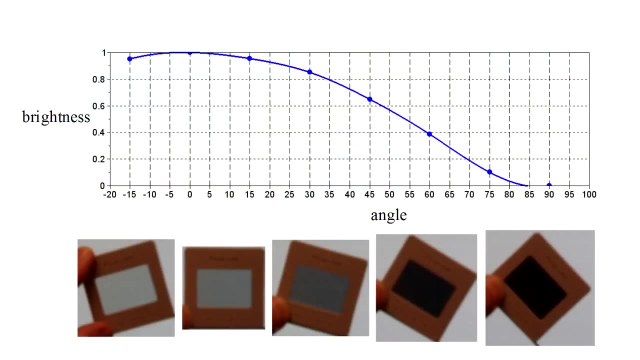 which we introduced in video 9.. When polarized light encounters a polarization filter, the emitted intensity depends on the filter orientation. Here's the relationship between transmitted intensity and orientation angle. I measured with my inexpensive webcam. Essentially, we'll use this result to test Bell's inequality, although for convenience. 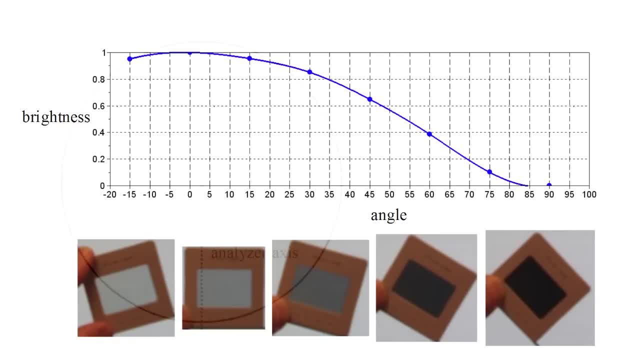 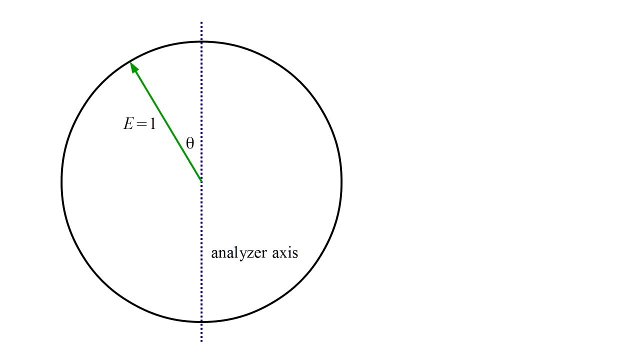 we'll work with the ideal theoretical form of this curve. A polarization filter operates as follows. Suppose an electric field is oriented at an angle, theta, to the filter axis. We can think of the field as having one component parallel to the axis, which varies as the cosine of theta and is transmitted by the. 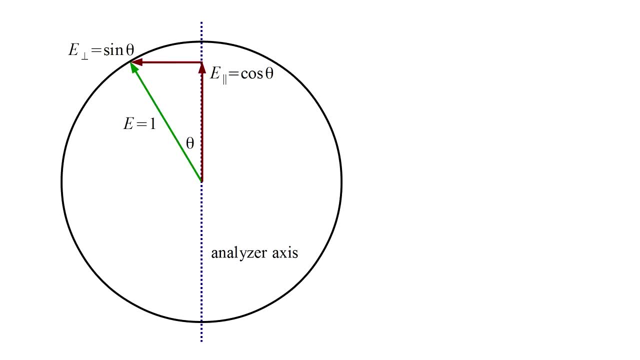 filter and another component perpendicular to the axis, which varies as the sine of theta and is blocked by the filter. The intensity of the transmitted field is the square of the transmitted electric field, hence cosine squared theta. The intensity of the transmitted field is the square of 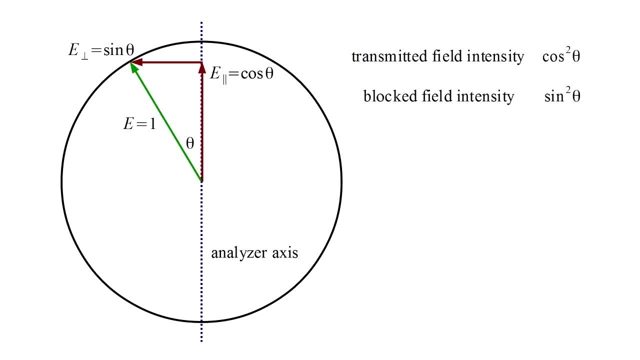 the transmitted electric field, hence cosine squared theta. The intensity of the transmitted field is the same, but we have to change that in order to convert it to zero. The intensity of the blocked field is likewise sine squared theta, Since a photon has to either completely pass the filter or be completely blocked under. 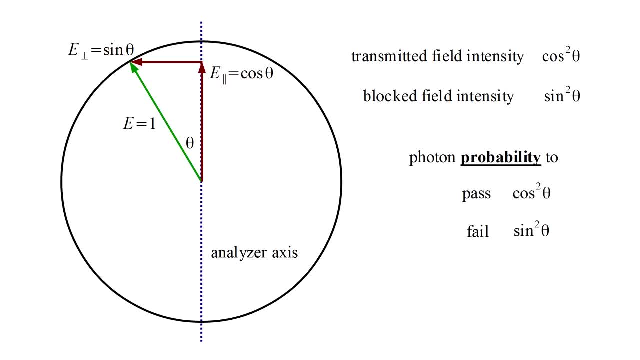 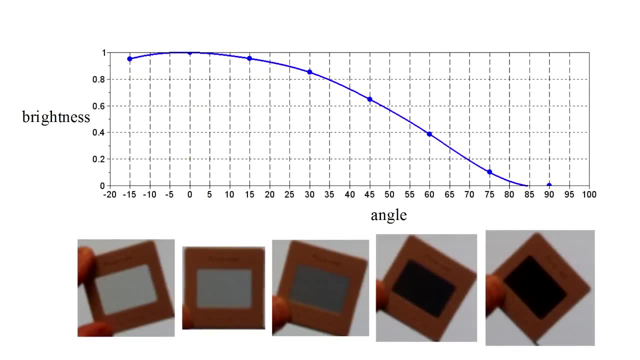 wave particle duality. we have to interpret these expressions as the probability for a photon to pass or fail to make it through the filter. Cosine squared of theta is the theoretical form of this measured curve, and sine squared is simply 1 minus this. 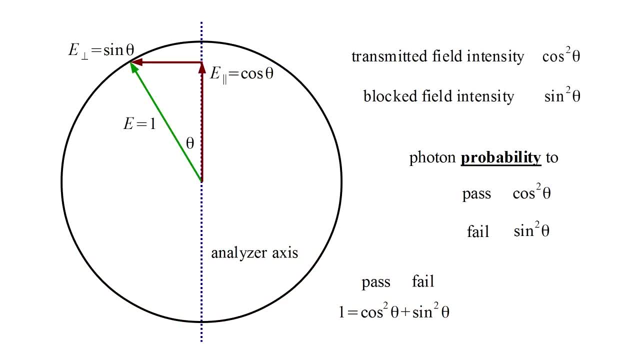 identity says: cosine squared theta plus sine squared theta equals one. This means that the photon either passes or fails with 100% probability. The average of cosine or sine squared over all angles is one half. The angled brackets here denote an average. This means 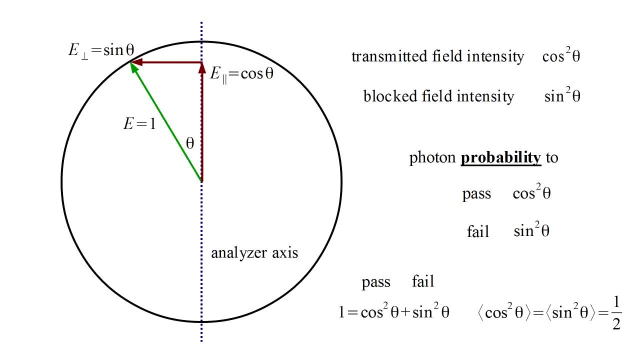 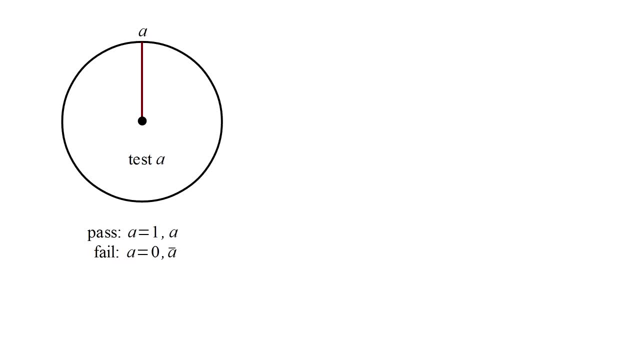 that randomly polarized photons will pass the polarizer with probability one half. Our three experimental tests are as follows: A filter with its axis oriented vertically forms test A. A filter rotated at an angle theta forms test B. And a filter rotated at an angle two theta forms test C. 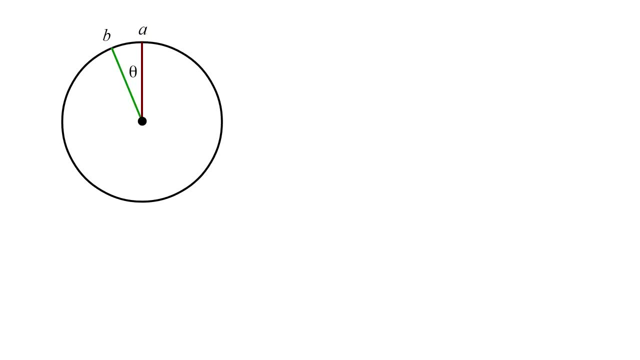 To test Bell's inequality, we combine tests A and B and look at the probability that a photon passes test A but fails test B. Assuming the photon is randomly polarized, it will pass test A with probability one half. Having passed test A, it must then be linearly polarized. 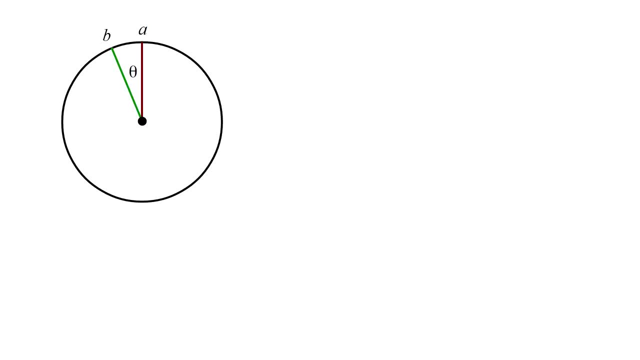 like this, Then the probability that it will be blocked by filter B, which is oriented at an angle theta relative to filter A, is sine squared theta. Therefore, the probability to pass A and fail B is one half sine squared theta. The same process for test B, followed by test. 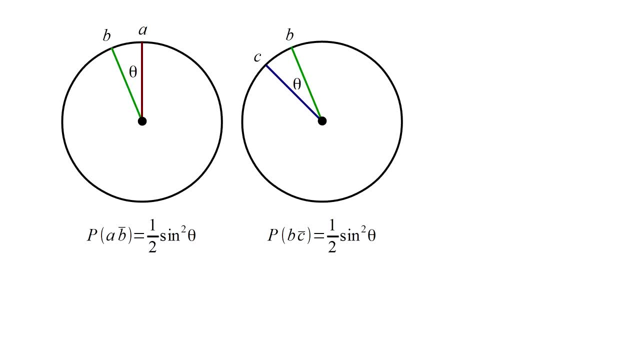 C gives the probability to pass B and fail C is also one half sine squared theta. Likewise, the probability to pass test A and fail B is one half sine squared theta. So we Hughes andsell them. Bell's inequality says that the sum of the first two probabilities should be greater. 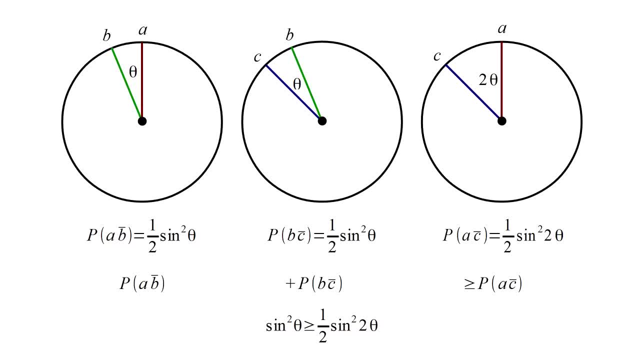 than or equal to the third. with one half sine squared theta plus one half sine squared theta results in real sine squared theta. So Bell's inequality says that sine squared theta is greater than or equal to one half sine squared of two theta. According to Bill兩ahel, underlying the equation B equals sine squared theta plus. 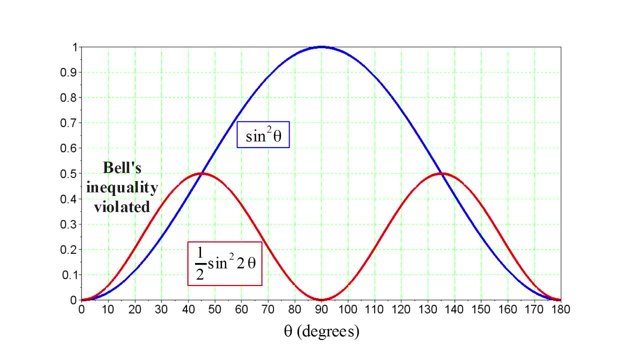 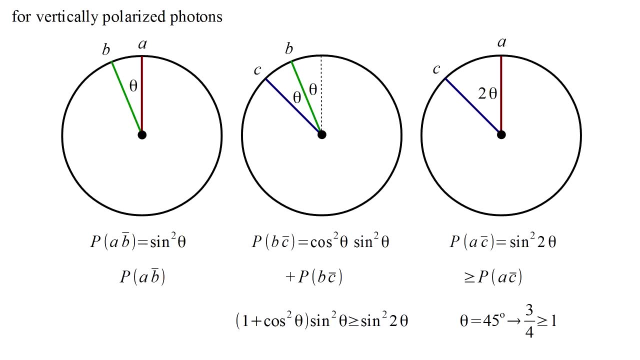 one quarter times sine squared theta. A plot of two extra quantities shows that this is not true for theta being plus eight times verbs between zero and 45 degrees, Bell's inequality is violated. If you're uncomfortable with the assumption of a randomly polarized photon, assume we use. 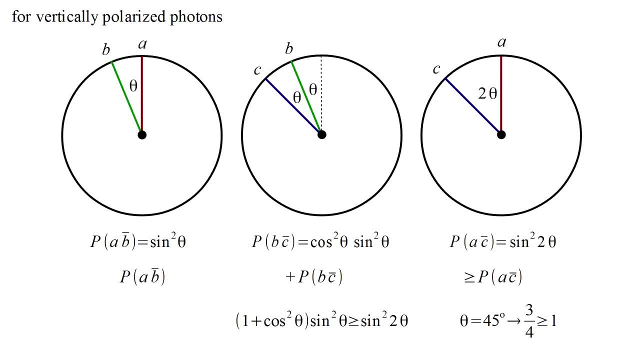 vertically polarized photons. The probabilities are then: sine squared theta, cosine squared theta, times sine squared theta and sine squared two, theta For theta equals 45 degrees. Bell's inequality reads: three fourths is greater than or equal to one, which is false. 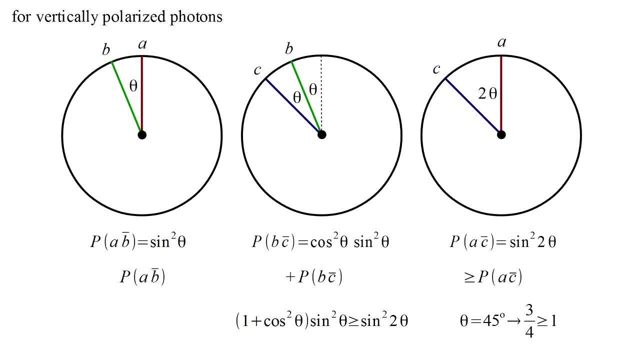 Now this is a profound result. so let's exercise some skepticism and really think about the details of how we would perform this experiment. We're going to assume ideal filters and detectors. In the real world, things are imperfect and typically additional steps need. 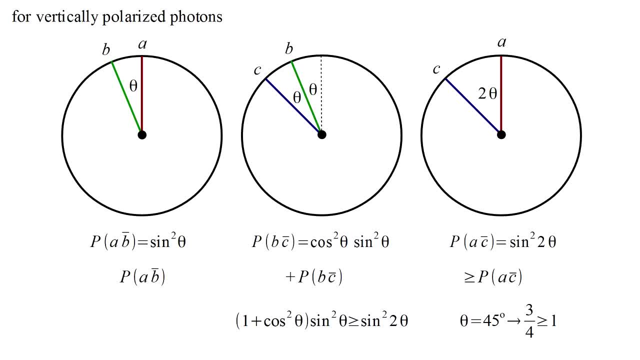 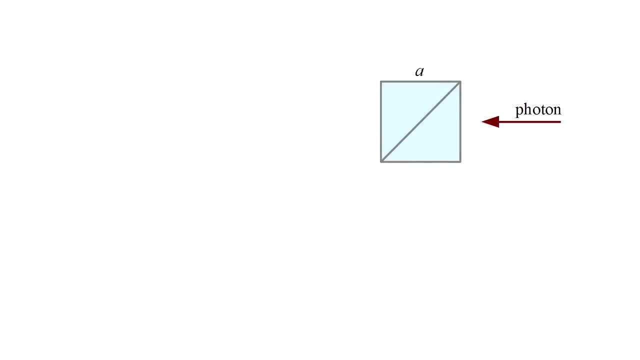 to be added to experiments and analysis. to compensate for this, Instead of simple polarization filters, we would want to use polarizing beam splitters. We discussed these in video 9.. If a beam splitter performs test A and the photon passes, then it continues on in a straight line. If it fails, instead of being absorbed. 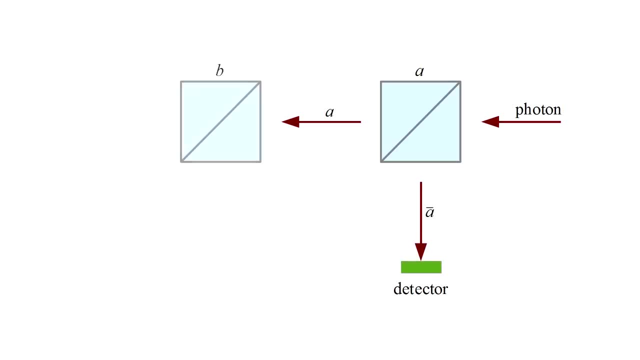 it's deflected and falls on a detector. If the photon passes test A, then it encounters a beam splitter for test B. If it passes, it continues in a straight line and strikes a second detector. If it fails test B, it's deflected and falls on a third detector. 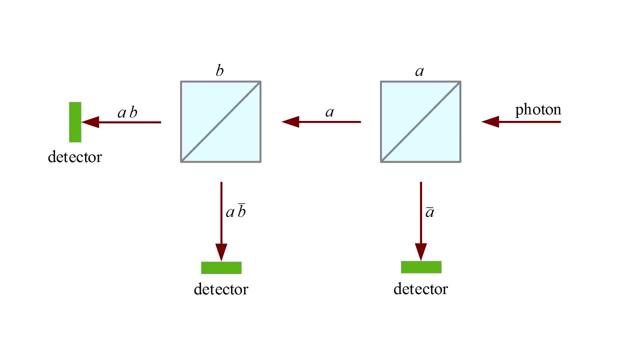 For every photon entering this system, one detector registers a signal. The fraction of those two signals produced by the middle detector is our measure of the probability of passing test A and failing test B. A similar setup can implement test A followed by test C. 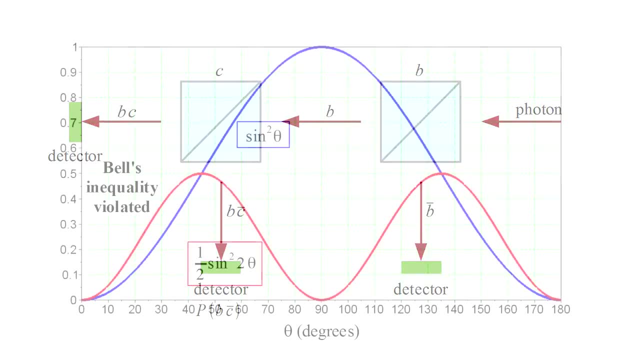 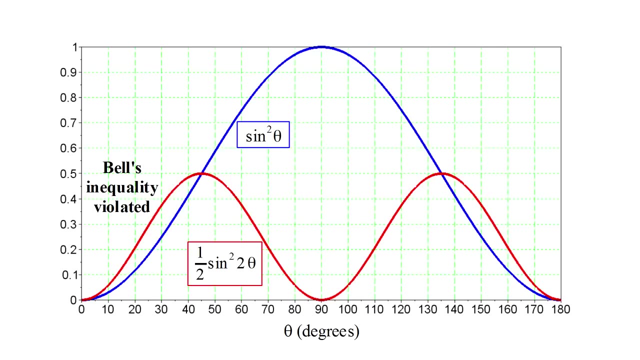 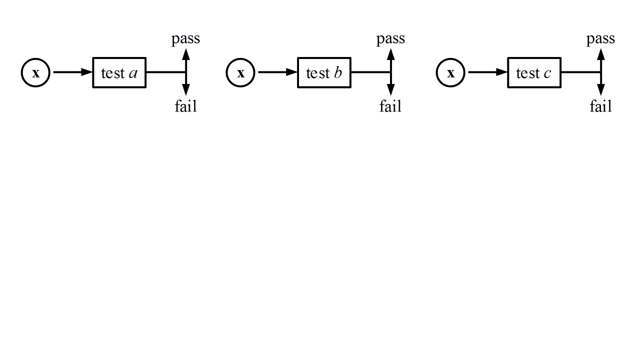 or test B followed by test C. Doing this will show the violation of Bell's inequality we've already discussed. However, there's a loophole In deriving Bell's inequality. we assume that the tests are performed on one or more particles in the identical state x. 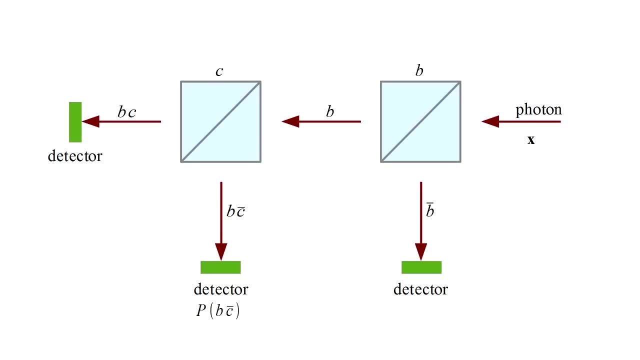 If a photon enters our device in the state x and passes the first test, can we assume that it's still in the state x when it encounters the second test? Let's remember Bohr's warning about the finite and uncontrollable interaction between the objects. 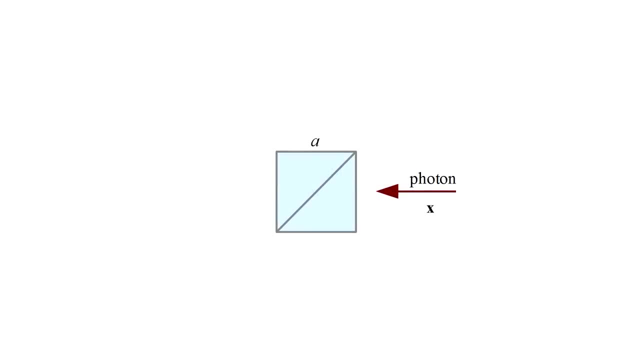 and the measuring instruments. Maybe a photon in state x that passes through a polarization filter comes out in a different state, y? If so, then we can't use that photon for additional measurements without violating the assumptions of Bell's inequality. In fact, we can show that this must be the case. 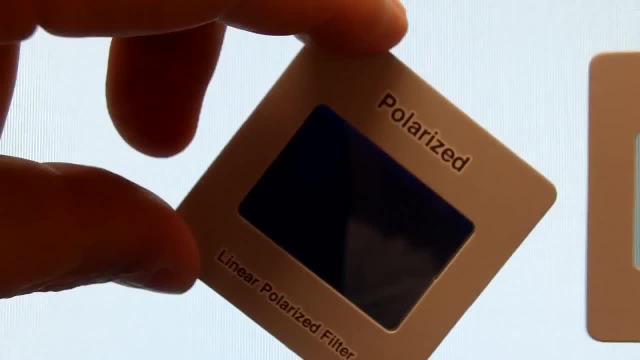 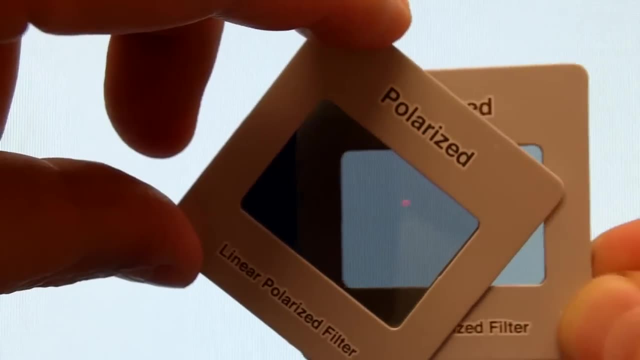 The light emitted by my LCD monitor is linearly polarized. Here I've oriented a polarization filter to block 100% of this light If we insert a second polarization filter. it will block 100% of this light If we insert a second polarization filter. however, 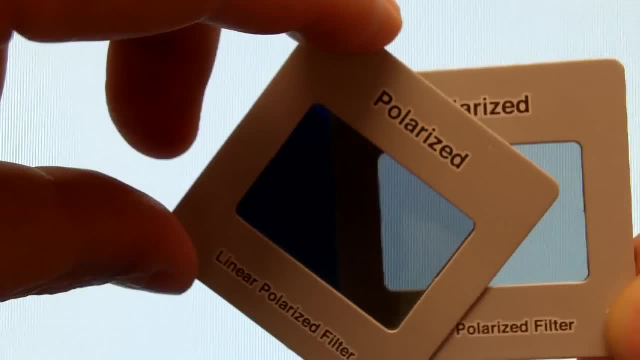 we can actually get some light to pass through both filters. Assume the photons emitted by this screen are in state x, As shown on the left, 100% of such photons fail to pass filter d. But, as shown on the right, if they first encounter filter c, some pass and subsequently go on to pass. 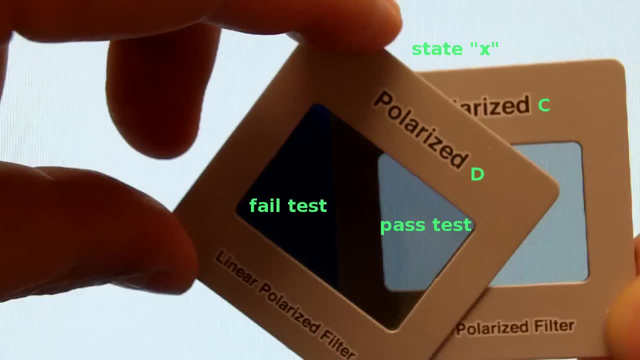 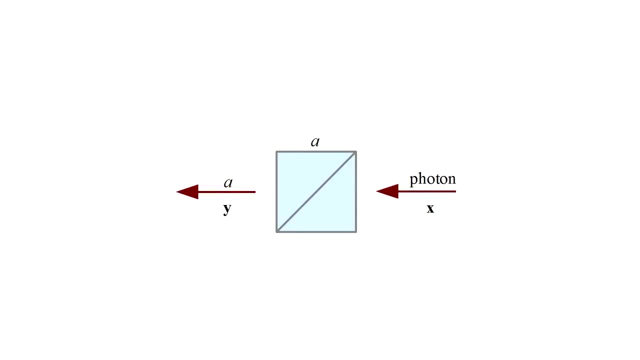 filter d. But if they eventually pass filter d they cannot be in the original state x, Because all photons in state x are blocked by filter d. They must come out of filter c in a state other than x. So when we measure the polarization state of a photon, 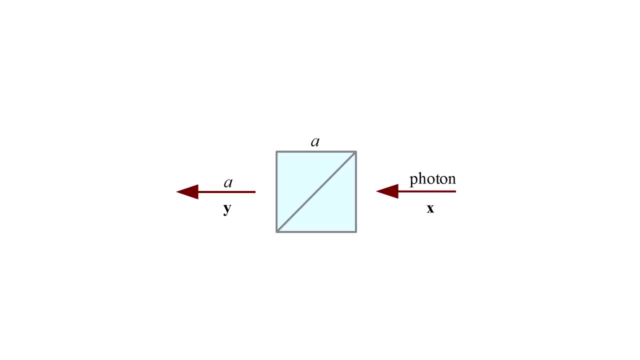 we cannot assume it ends up in the same state that it started in. Well, did we just waste several minutes? No, we're going to fix the loophole and this will all tie together. But first let's go back to our cartoon experiment. We might imagine that as a 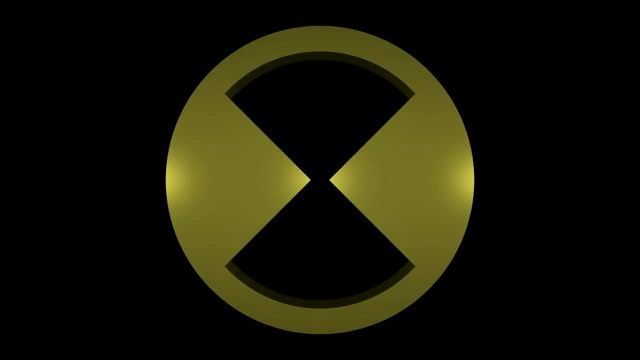 copper bar is passing through a brass disk, it experiences some interaction that changes its state, its orientation. Consequently, performing two tests on the same bar may not give us the same results we would have obtained without the interaction, or that we would obtain from. 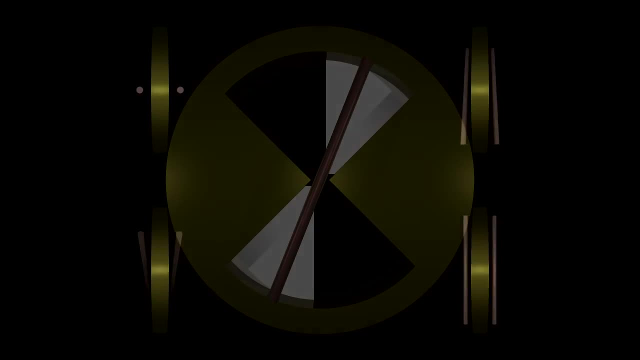 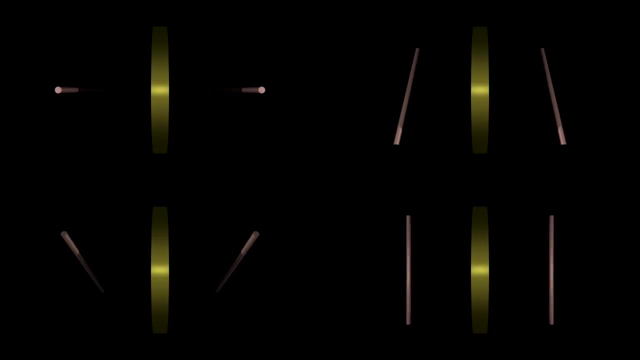 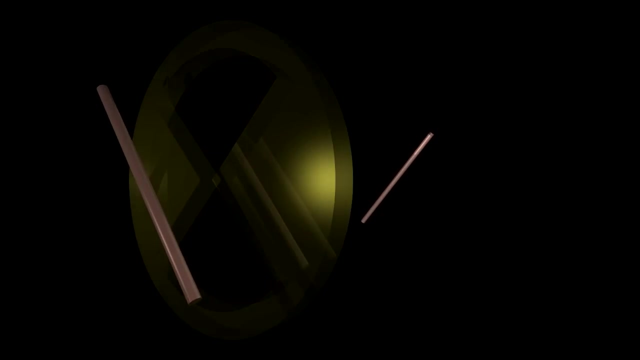 independent tests on identical bars. But suppose our copper rod source produces two rods traveling in opposite directions at the same angle x. Now if a measurement on one rod changes its state, we have a copy for the second test. We'll run our two tests on the two identical rods. 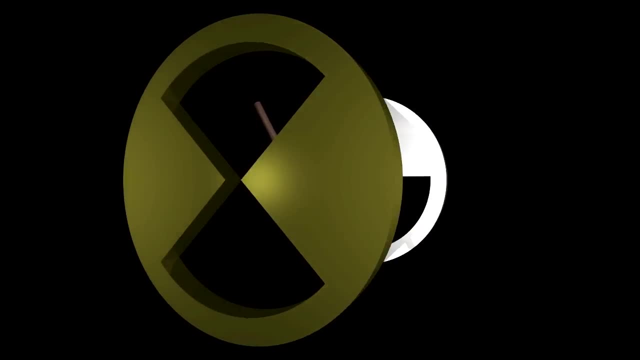 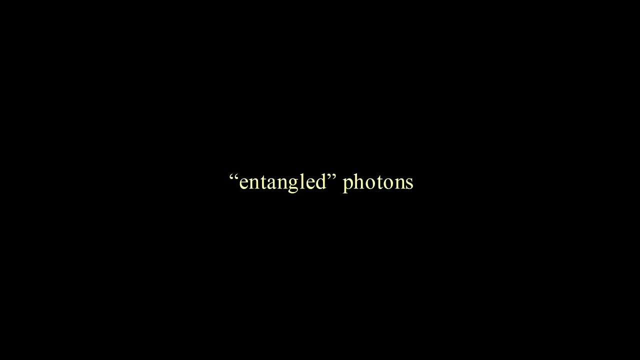 Because no rod is used for more than one test, we no longer have to worry about changes of state due to a measurement interaction. A real-world version of this takes the form of so-called entangled photons. One of the first proposals for generating entangled photons was through the decay of positronium. Positronium is 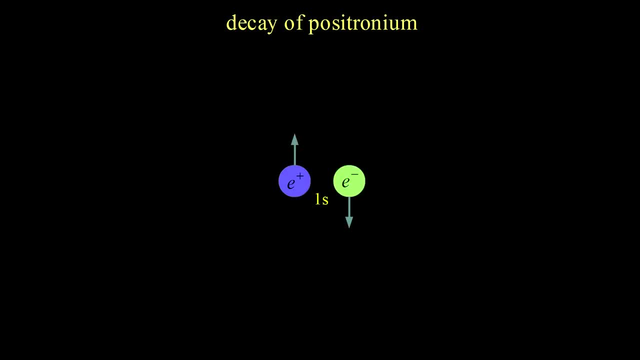 similar to a hydrogen atom, but with the proton replaced by a positron, the electron's antiparticle In the lowest energy state. positronium, like hydrogen, has no orbital angular momentum. If, in addition, the positron and electron spins are oppositely oriented and the atom 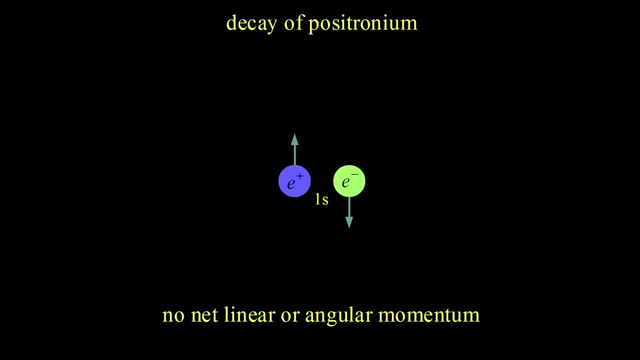 is at rest, there is no net linear or angular momentum in the system. Eventually, the antiparticles will annihilate each other and radiate two photons. In order for the photons to have no net linear or angular momentum, they will have to have 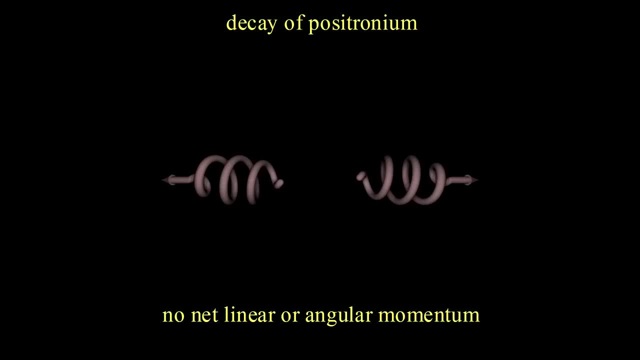 the same wavelength, travel in opposite directions and the angular momentum due to the combined spins will have to be zero. If, for example, one travels to the left with right hand polarization, the other will travel to the right with right hand polarization. Their angular momentum vectors point in opposite directions and cancel out. 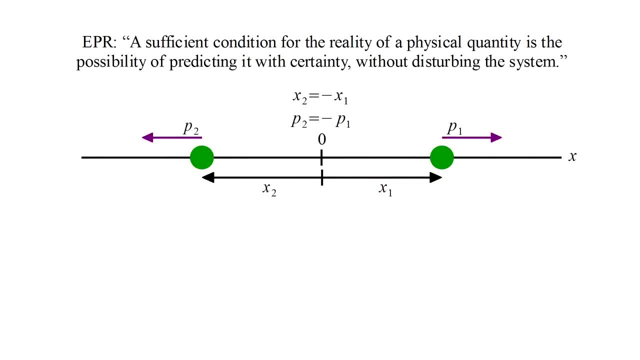 This creates a scenario very analogous to the Einstein, Podolsky and Rosen thought experiment. Actual experiments employ more complicated but more practical methods for generating entangled photons, but the basic idea is similar. The experimental evidence that the two photons are entangled comes from subjecting both to 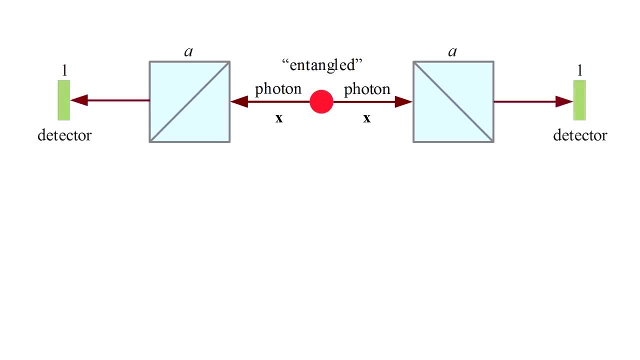 identically oriented polarization measurements. If one and zero represent pass and fail, then each photon generates a pattern of zeros and ones. The two patterns, although random, are identical. If the two photons were generated in different states, they would be identical. 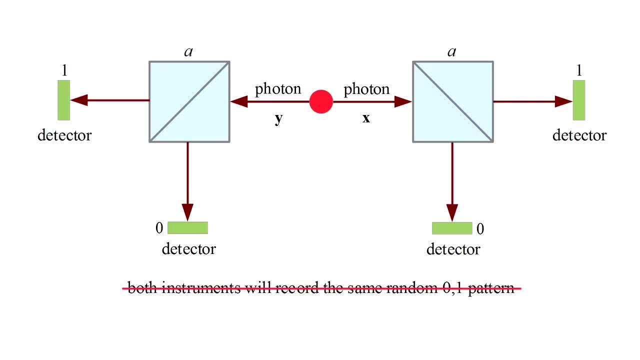 If the two photons were generated in different states, they would be identical. If the two photons were generated in different states, we would not observe this. At least some of the time. the patterns would be different. In fact, this is so reliable that it is used in the field of quantum cryptography to generate 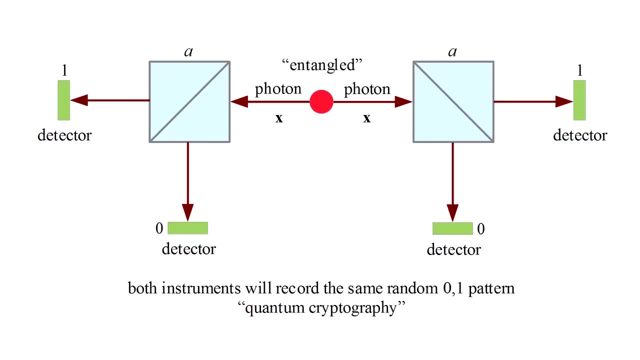 a shared random key for two users. The beauty is that for a third party to intercept the key, they'd have to detect one of the photons which destroys it and that will then be noticed by the intended users. To test Bell's inequality, we subject the two photons to different methods. 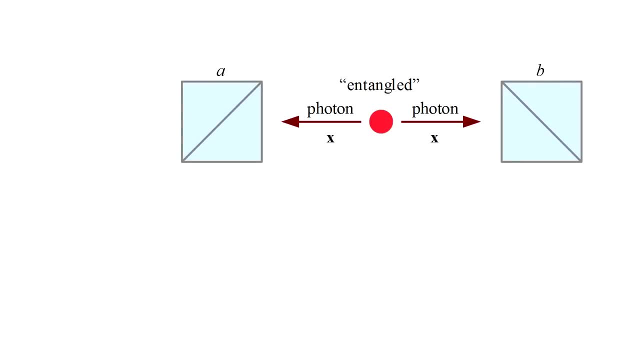 To test Bell's inequality, we subject the two photons to different methods. By counting the fraction of the time that the A and Not-B detectors generate coincident signals, we can measure the probability of A and Not-B. This has been done with a large separation between the photon measurements. 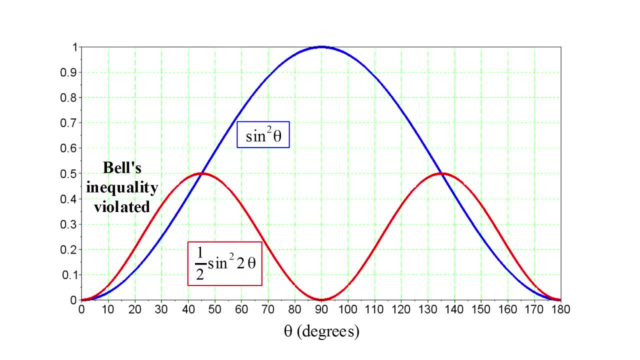 Experimental results consistently show that Bell's inequality is violated, just as in the single photon scenario. We could explain this away when using a single photon to perform two experiments- In this case it was a single photo and a single photon- The Driver's Inequality is not quantized to the temperature that is being measured. 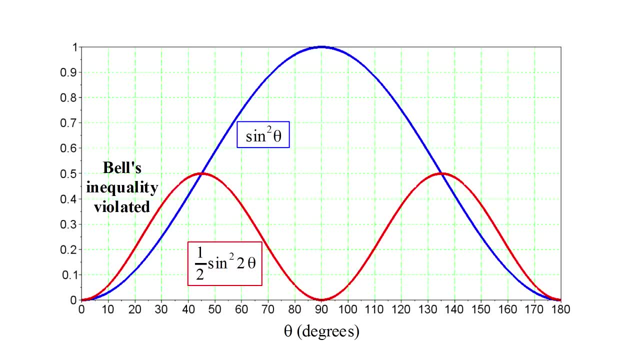 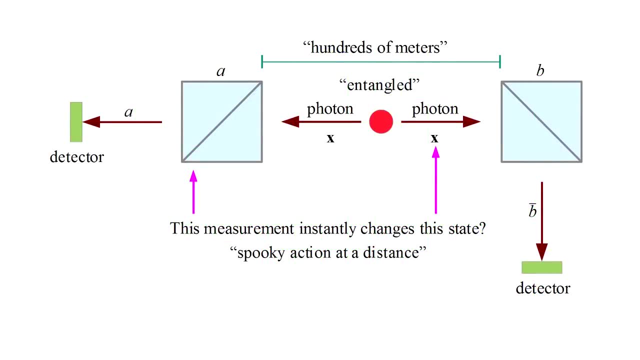 perform two tests. The first measurement changed the photon's state, so the second measurement didn't conform to the assumptions of Bell's inequality. But if we want to use that explanation for the entangled photon version, then we have to assume that a measurement on one photon instantly changes the state of the other photon. 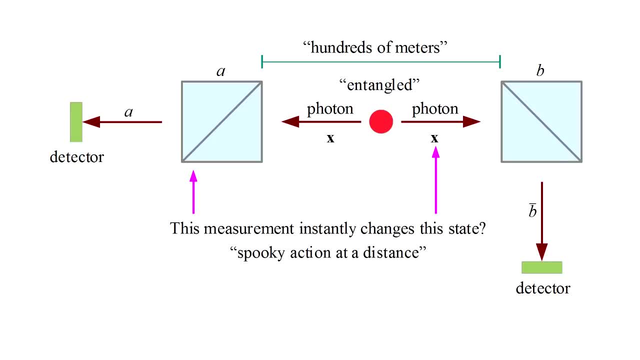 The change has to be instant, because the two measurements can be arranged to be arbitrarily close in time. Indeed, if they're simultaneous, then we'd have to ask which measurement was influencing the other. This is precisely the picture that the EPR paradox found unacceptable. where reality 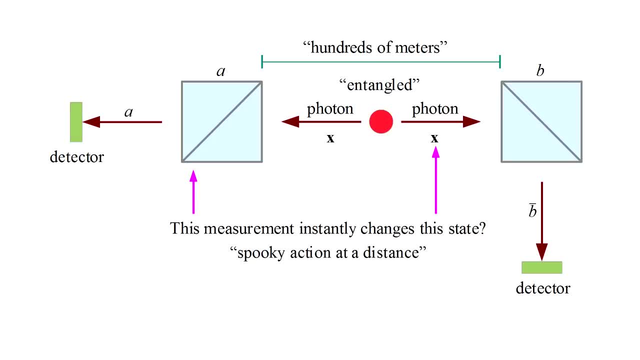 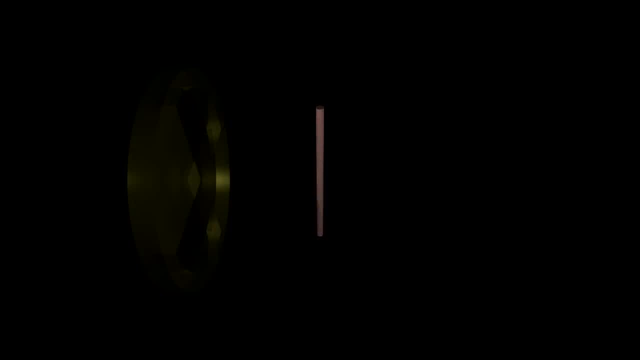 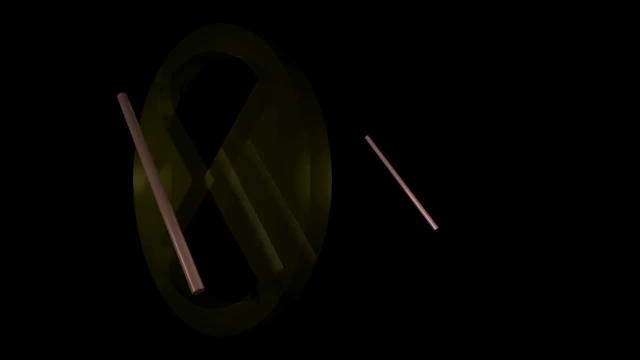 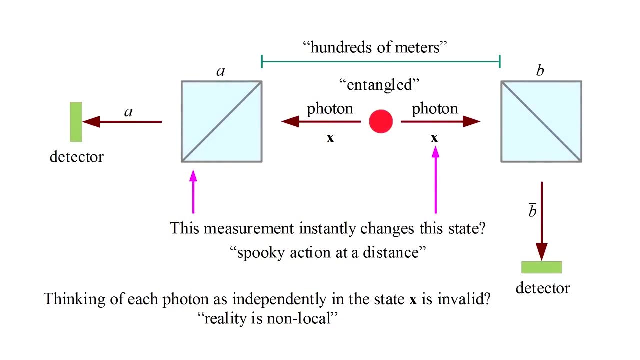 for one particle depends instantaneously on a distant event, what Einstein referred to as spooky action at a distance. In our cartoon experiment, we might visualize this as a measurement on one rod, causing both rods to simultaneously change their state. Alternately, maybe thinking that each photon is independently in a state X is invalid. 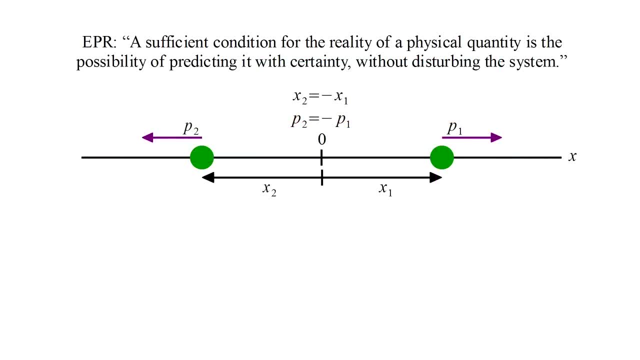 Reality in this sense is non-local. Indeed, this gets to the heart of Bohr's response to the EPR paradox. EPR stated �A sufficient condition for the reality of a physical quantity is the possibility of predicting it with certainty without disturbing the system� Implicit in the thought experiment. 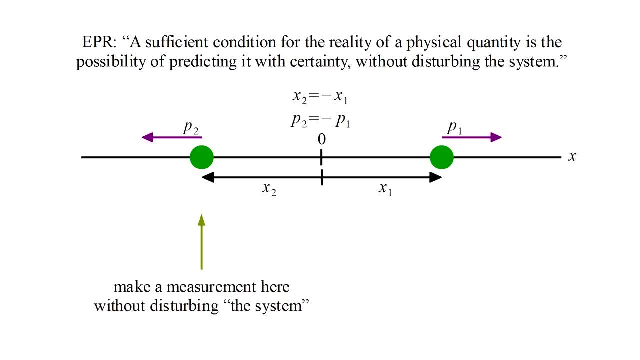 was the idea that the primitive density é was the density of the outside air. at the that one can measure the position or momentum of particle two without disturbing the system. The system, in this view, is particle one, But quantum mechanics requires that the system 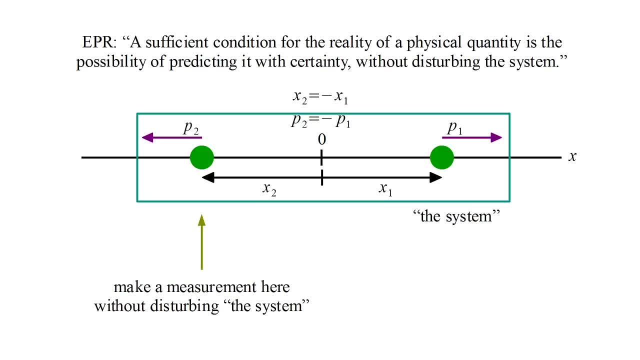 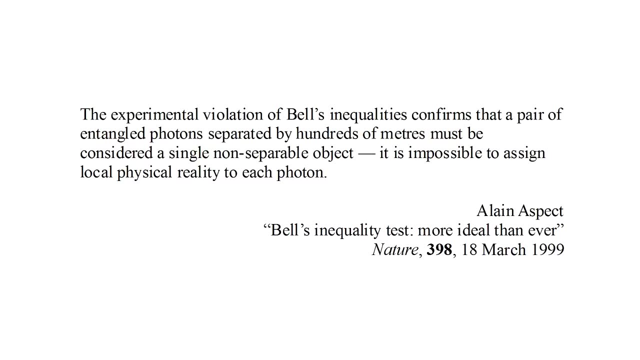 include both particles which together are described by a single wave function. It is not possible to make a measurement on either particle without disturbing the entire system. This is the ambiguity in the EPR definition of reality which Bohr pointed out. As stated by Alan Aspay, the experimental violation of Bell's inequalities confirms. 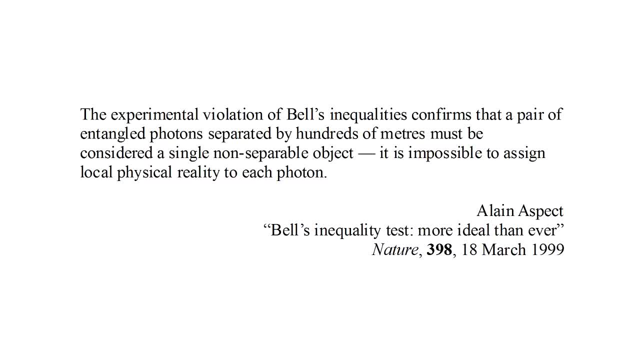 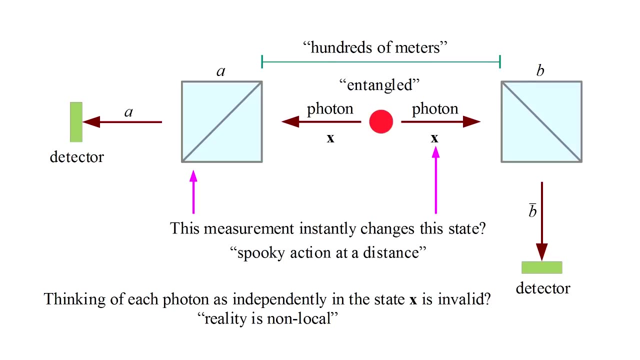 that a pair of entangled photons separated by hundreds of meters must be considered a single, non-separable object. It is impossible to assign local physical reality to each photon. The experimentally confirmed predictions of quantum mechanics are very clear and fundamentally incompatible with our common conception of locality.